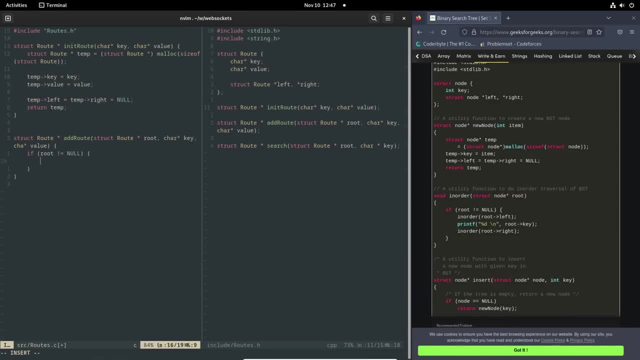 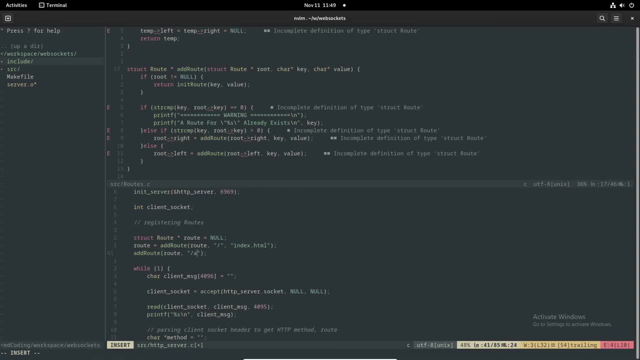 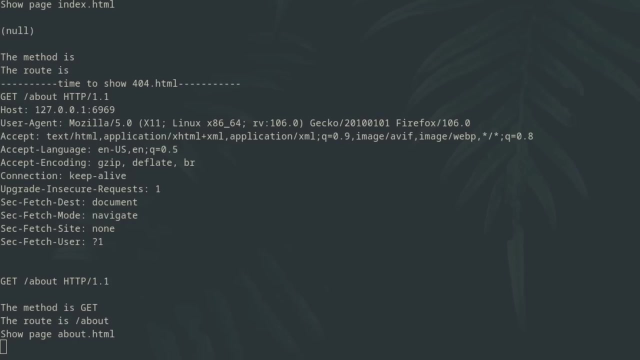 I used a BST because I didn't want to write my own map. After that, I tried using the route map in my main application and registered a couple of routes And, as you can see, it can now detect which route is being requested and then show the. 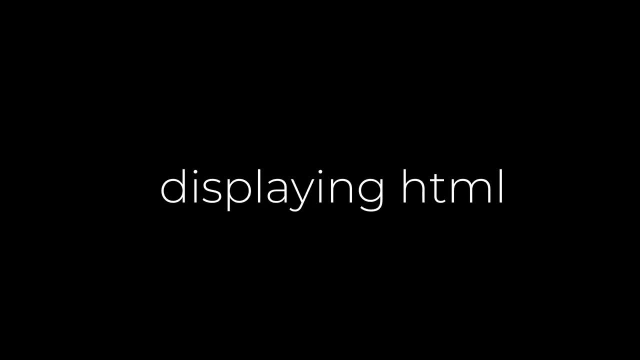 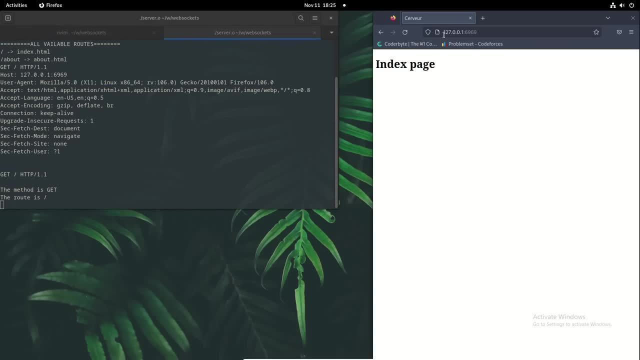 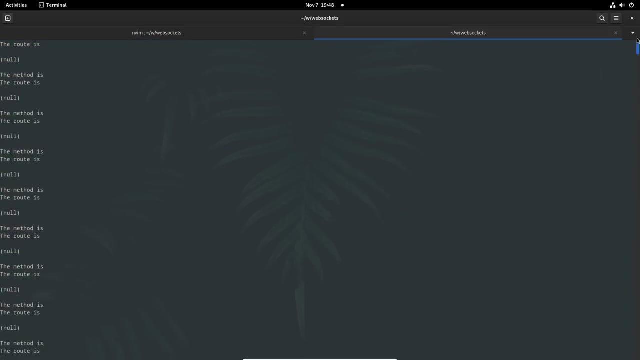 name of the corresponding HTML page. Then I wrote some code to display the actual HTML file and you can see that in action right now. So, yeah, that is pretty much it for this video. I know it's not really that much, but I got the basics done. 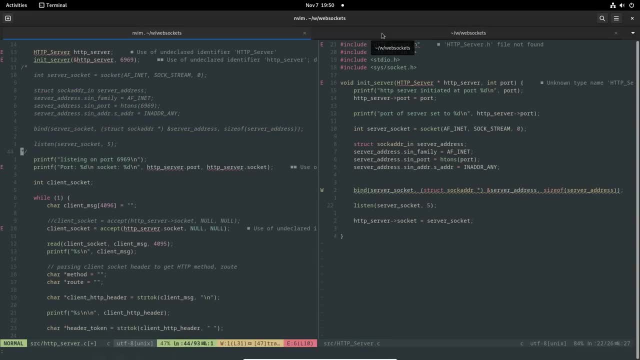 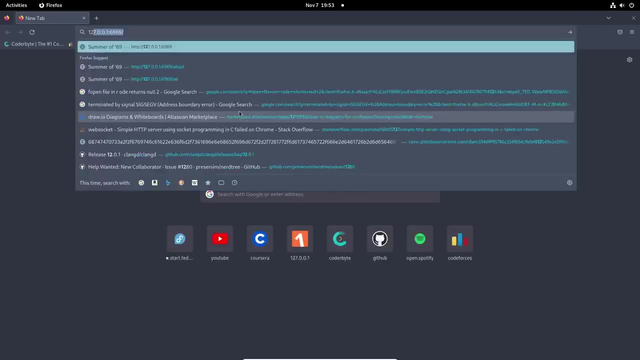 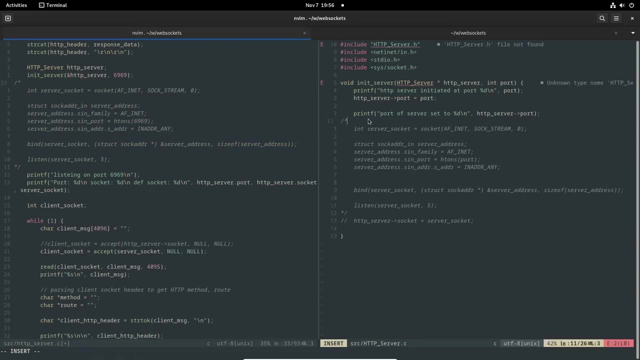 So basically the routing and showing the pages and stuff. And yeah, I got a lot of stuff to do parsing JavaScript and CSS and probably making some backend logic so connecting with database and stuff. But yeah, This is all I have. 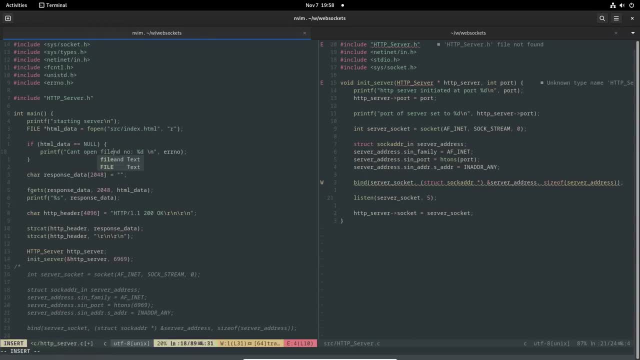 I will probably continue working on this project And, yeah, Let's see how far we can take this. 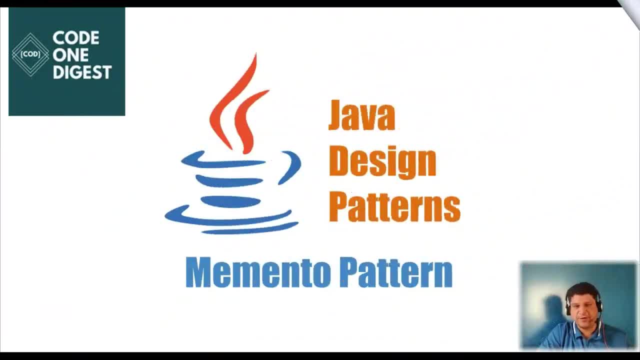 Hello, good morning friends. Welcome back to your favorite channel Code One Digest. In this video we will discuss what is Memento Design Pattern, Where to use Memento Design Pattern in our project. I'll also show you the Java code implementation of Memento Design. 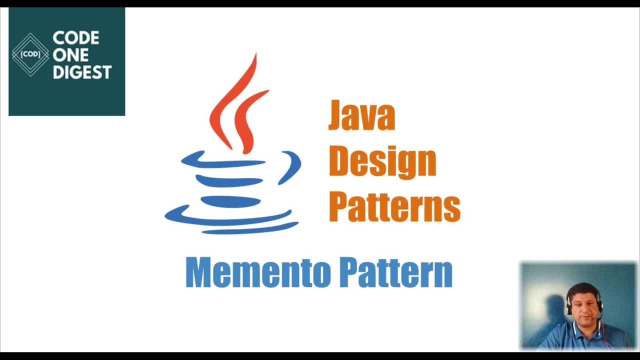 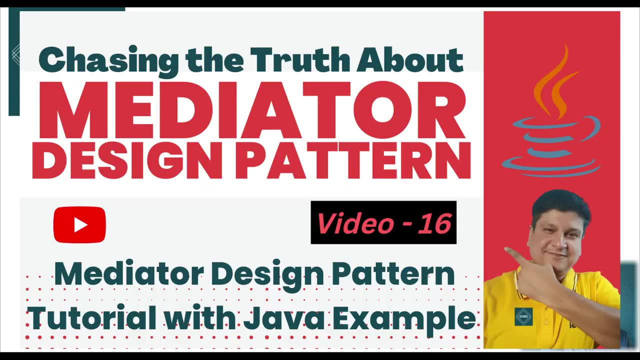 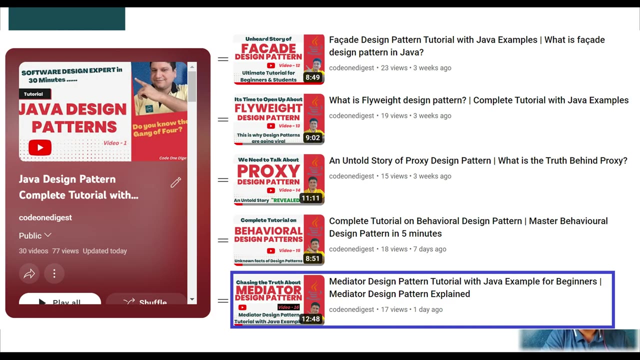 Pattern And at the end we will discuss the benefit of Memento Design Pattern. So stay tuned till end of the video, Friends. in the previous video we discussed about Mediator Design Pattern. Can you explain what is Mediator Design Pattern and where to use it, Please? 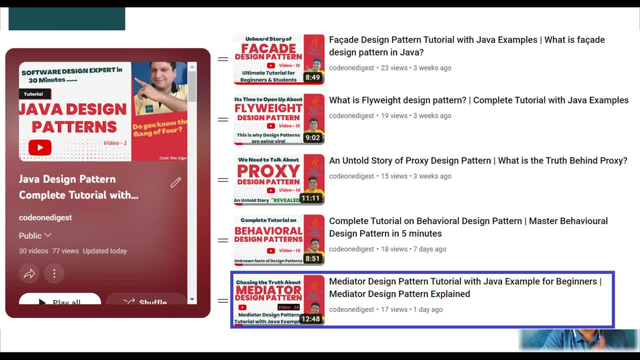 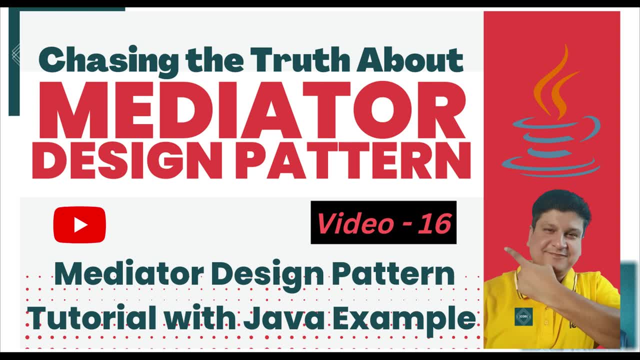 reply your answer in the comment section And if you have not seen the previous video, I'll recommend you to go and see that video. That's very important video and design pattern. The link is provided on your screen and also given in the description section. And just.